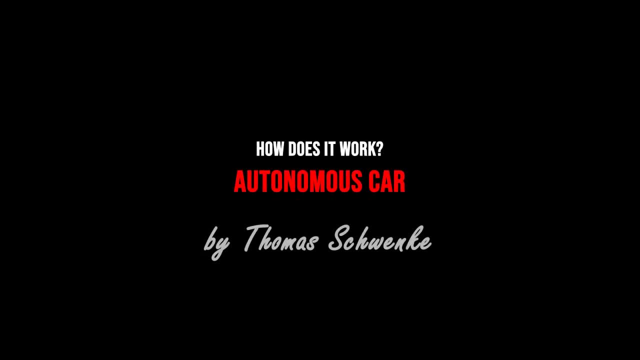 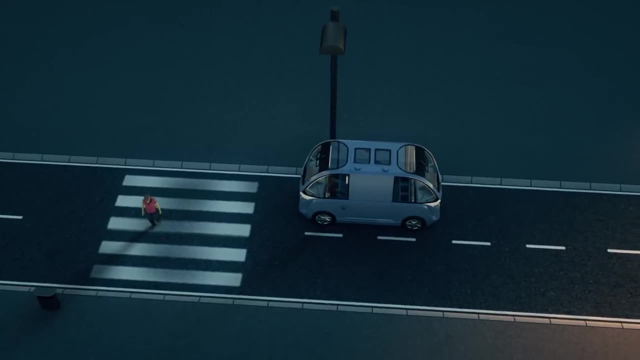 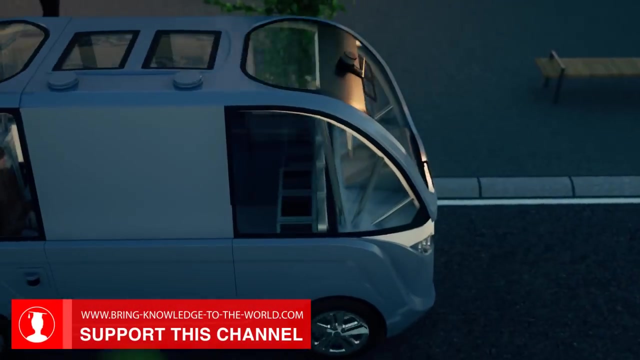 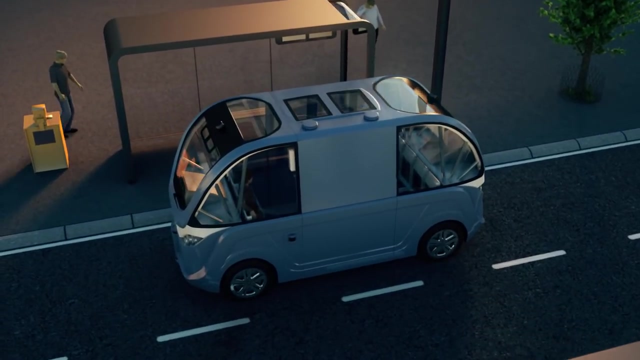 Self-driving vehicles can detect obstacles and stop if necessary. With the help of sophisticated technology, vehicles from Navaya, Waymo and local motors are able to pick up passengers on demand and take them to their desired destination. Autonomous vehicles are also able to recognize traffic lights and road signs at intersections. 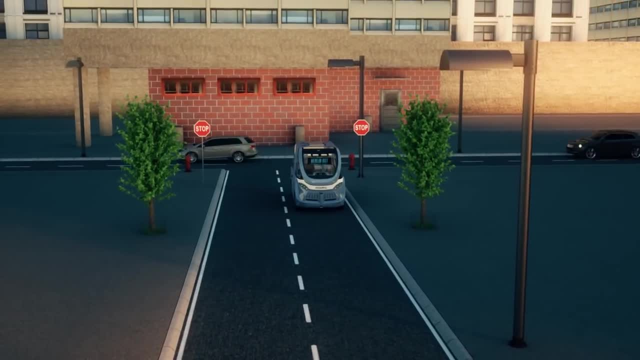 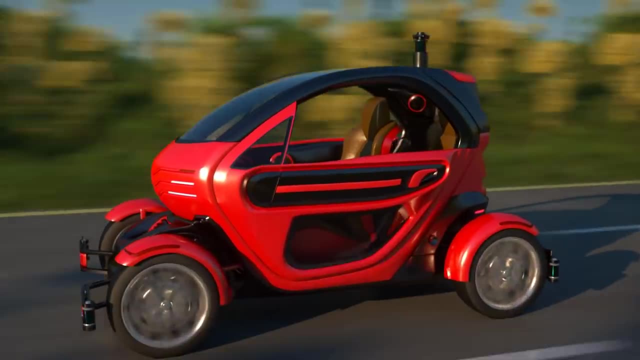 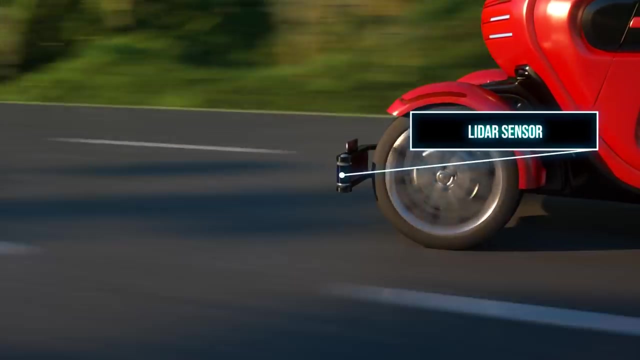 and act accordingly, But how do they actually do all this? Self-driving cars do not require a driver to get from A to B. The technology in and on the vehicle is the driver. The technology includes many sensors, such as LiDAR sensors, ultrasonic sensors, cameras and radar sensors. 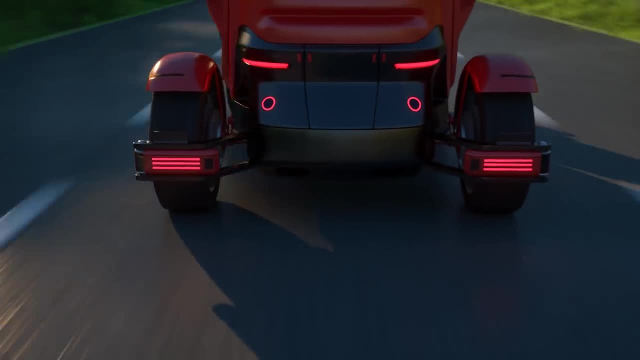 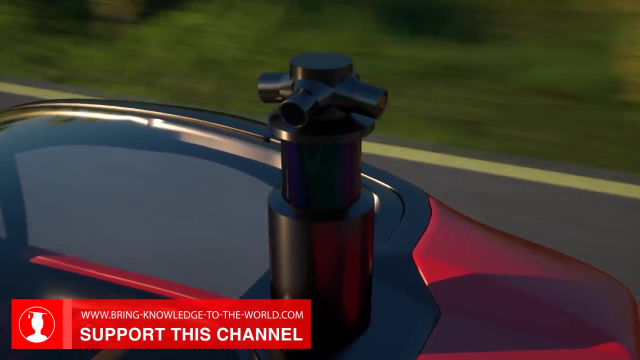 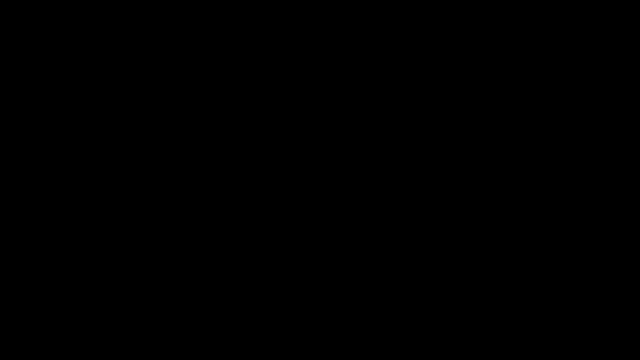 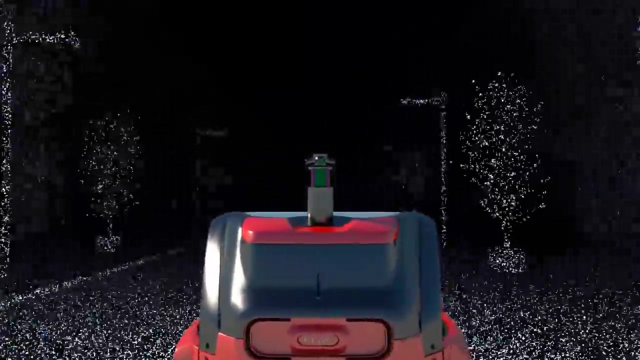 The sensors are located at the front and the rear of the vehicle. Cameras and LiDAR sensors are also frequently found on the roof. Without them, the vehicle would be virtually blind. LiDAR is a key component in many vehicles. LiDAR works similar to radar. 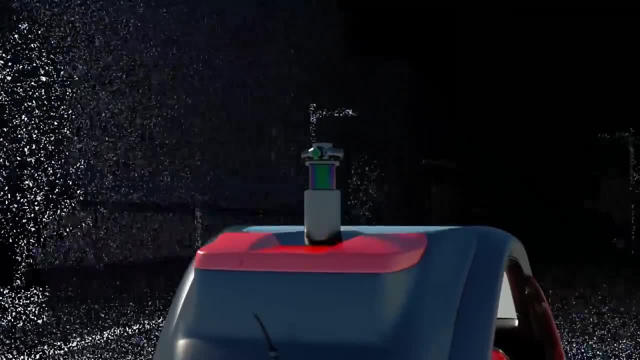 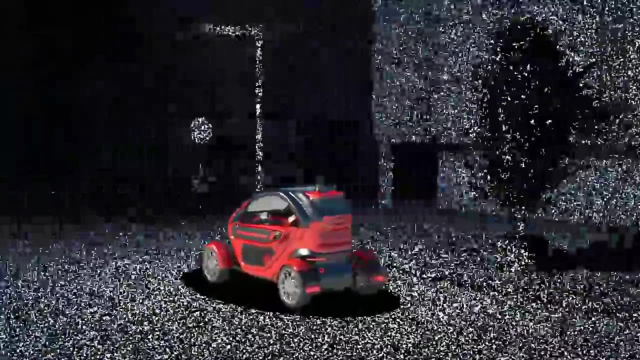 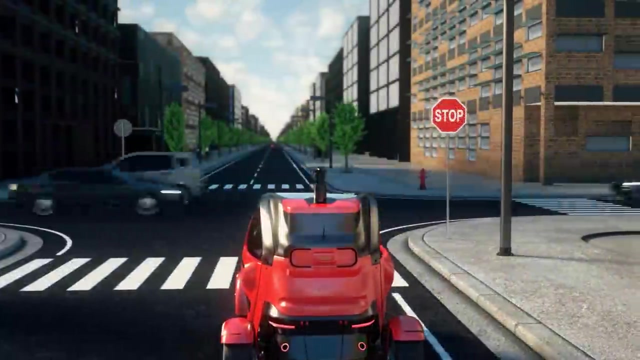 LiDAR, however, does not use radio waves, but many light rays that are reflected by the objects in the surroundings and detected by the LiDAR sensor. In this way, a point cloud is generated. However, LiDAR does not recognize road signs. 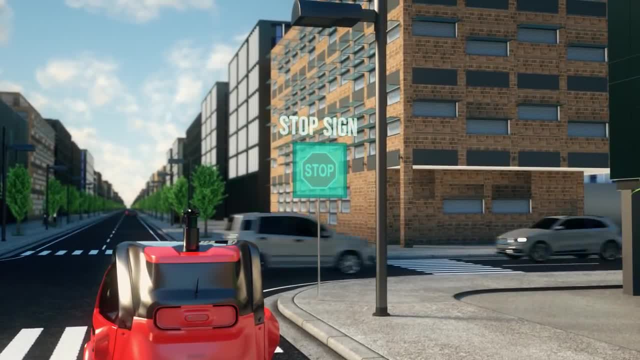 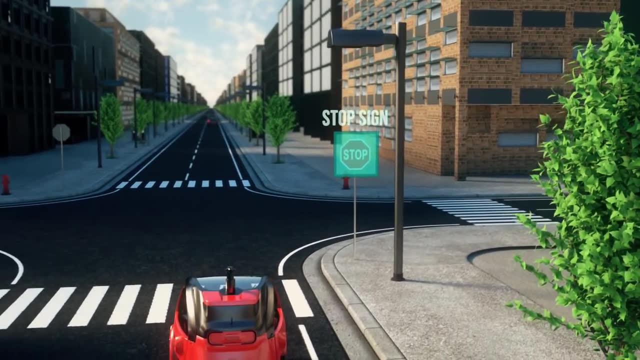 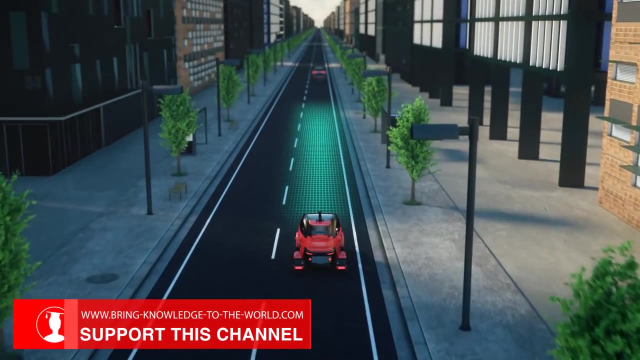 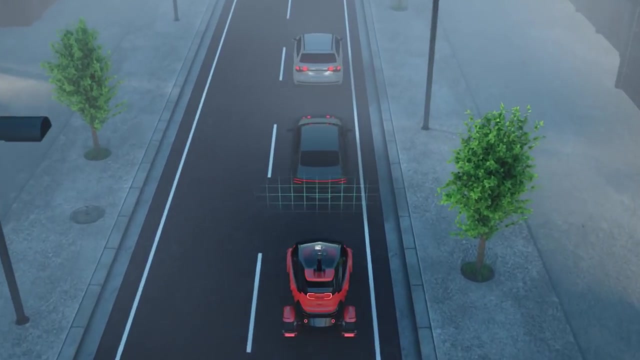 Cameras use artificial intelligence to recognize and interpret street signs. Cameras are also used to detect obstacles and are needed for lane keeping. Neither LiDAR nor cameras can handle fog. In this situation, radar is needed for forward collision warning and avoidance. A major disadvantage of radar, however, is that the objects must be large enough to be detected. 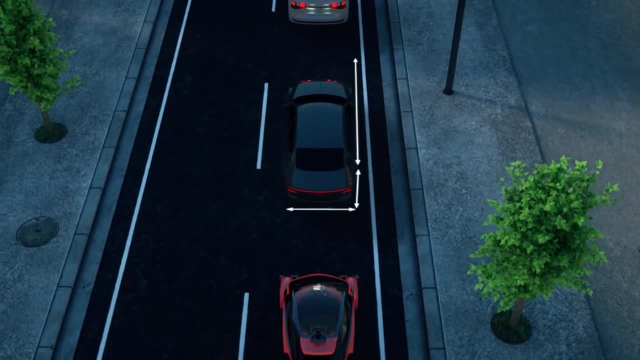 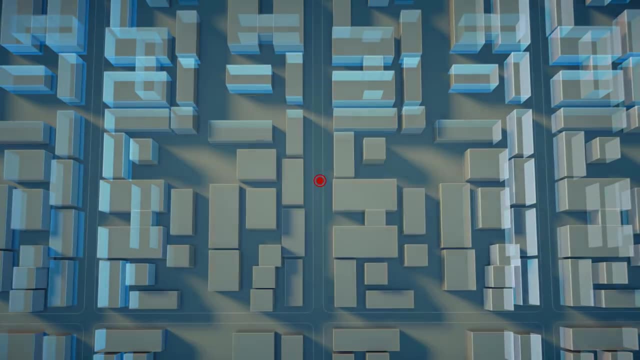 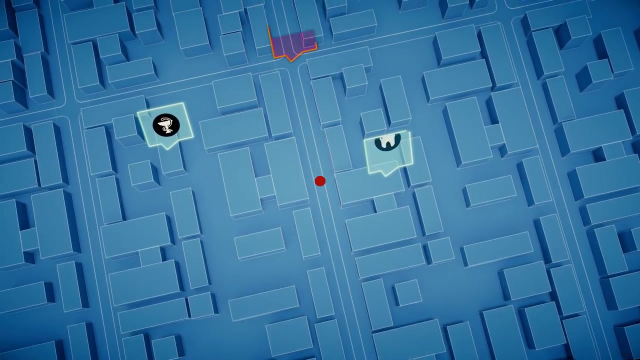 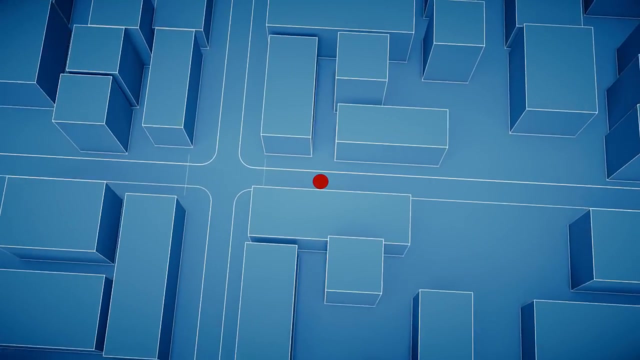 Pedestrians or cyclists may therefore not be recognized by radar. The exact position of the vehicle is determined by GPS and highly accurate digital maps. Digital maps contain a lot of information, including information such as intersection signs and speed limits. Since GPS cannot always be guaranteed, for example, in tunnels and street canyons, odometry is also necessary.